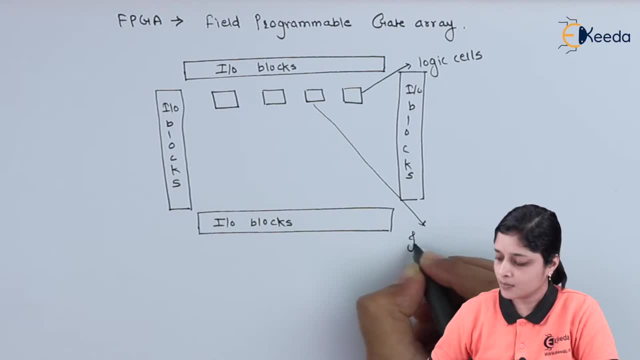 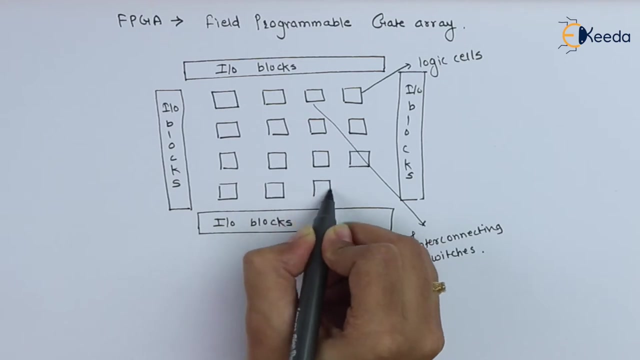 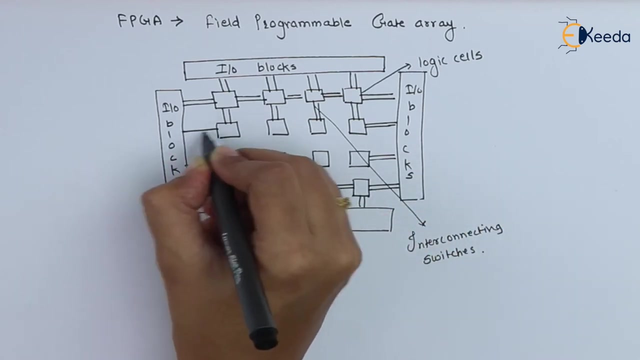 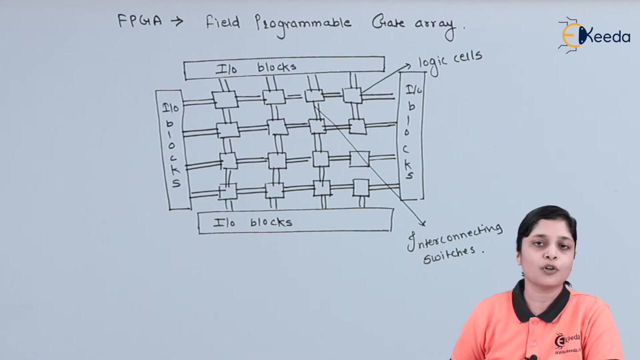 and VLSS Interconnecting switches. So we will draw logic cells and interconnecting switches alternately. We have to show here the interconnection between each and every block, So this becomes the block diagram for FPGA. Now the important point regarding the FPGA is: it is a VLSS circuit. 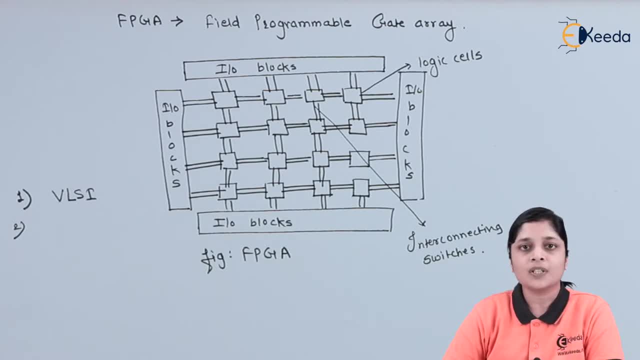 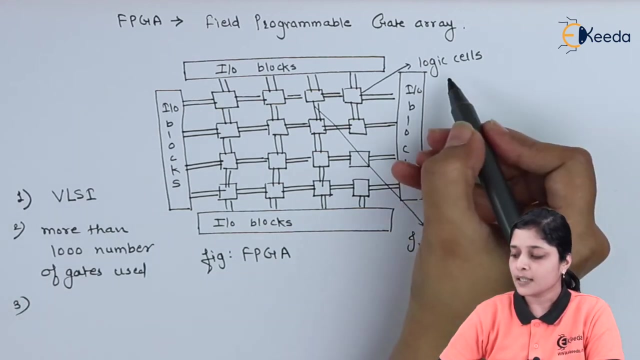 Means more than thousand number of gates. you can implement a VLSS circuit, So this becomes the block diagram for FPGA. You can implement on single ICs According to the application you can use the number of gates. Now it consists of logic cells and interconnecting switches. 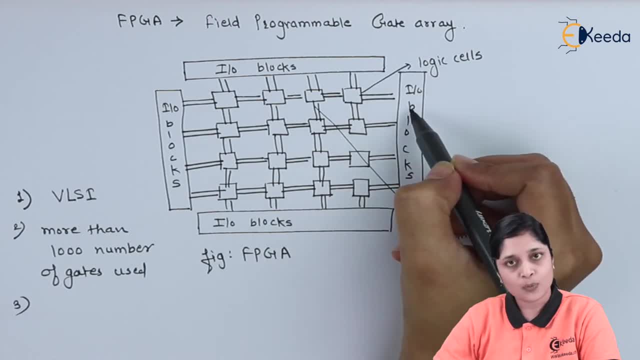 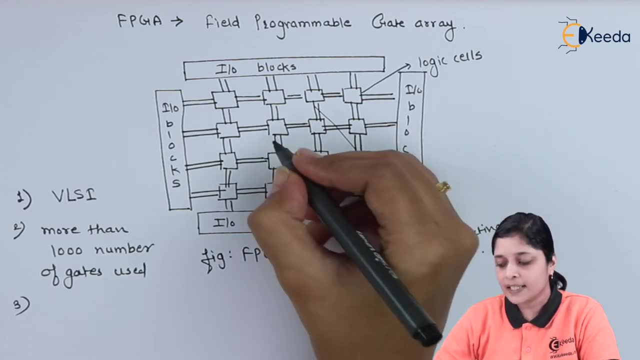 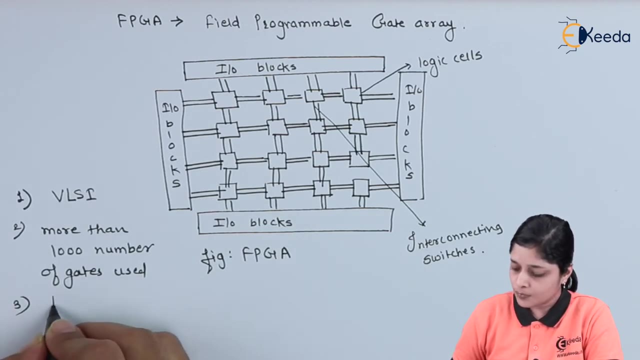 The interconnection between logic cells and IO block is programmable. Also, interconnection switches are used for interconnecting each and every block to get the desired output. So logic cells and interconnection between them is programmable. So this is all about the basic and important points regarding FPGA. 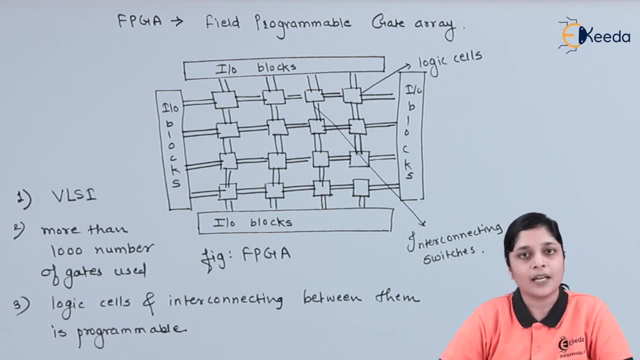 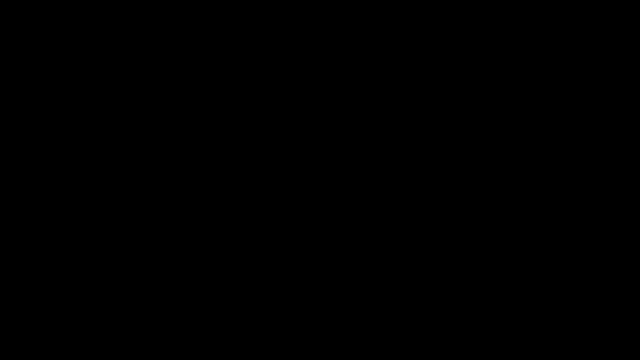 That is filled. programmable gate arrays. Thank you for watching this video. Stay tuned with IKEDA and subscribe to IKEDA. Thank you for watching IKEDA- IKEDA.